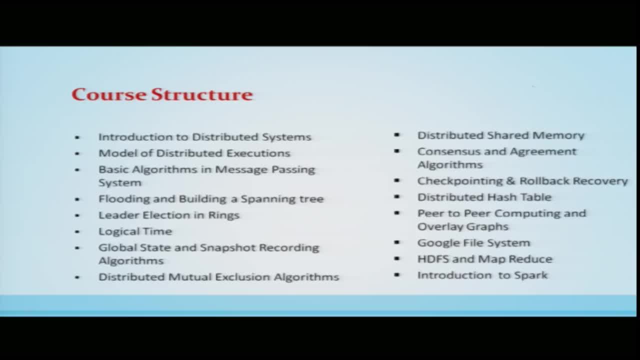 The course structure of a distributed system goes like this. So this particular course, if you see, is divided into two different parts. The first part is the perspective from the systems perspective- distributed systems. The second part is called distributed systems from algorithms perspective. 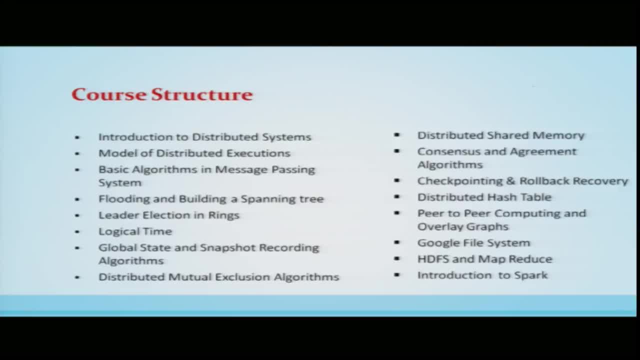 So the algorithms which will run on this model of a distributed systems is required to be understood here, So model also is required to be understood. and then the algorithms: how to design these algorithms, how to analyze it and different intricacies of this algorithm design. in this, 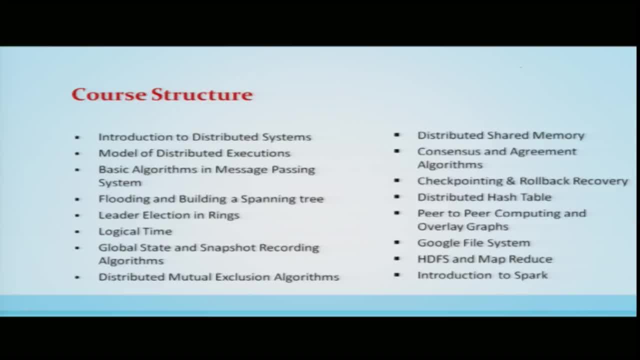 particular problem setting. So the main topics which we are going to focus on from algorithms perspective is how to build the spanning trees using flooding algorithms, then the leader election algorithm. These are basically most of the important algorithmic design techniques. They are the basic building blocks of the distributed systems. 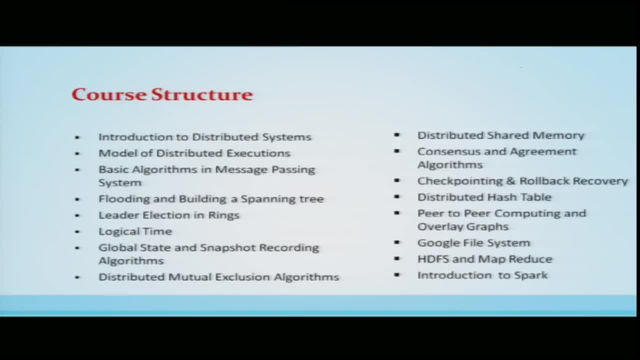 From systems perspective, we are going to cover up the global state recording, mutual exclusion, consensus, shared memory, checkpointing, rollback, distributed hash table and the case studies of a distributed systems, which we will cover here in this part of the course. structure is peer-to-peer Google file system, HDFS and introduction to the SPARC. 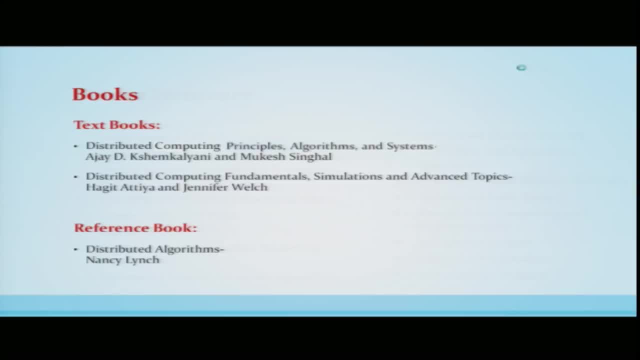 With this particular course, we will use two tools. First of all, we are going to talk about how to build a distributed system. Second of all, we are going to talk about how to build a distributed system. There are two text books. 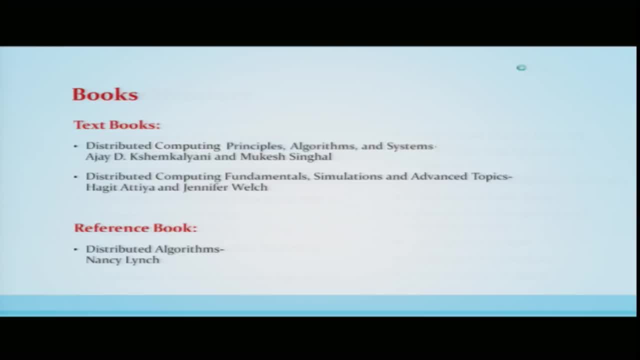 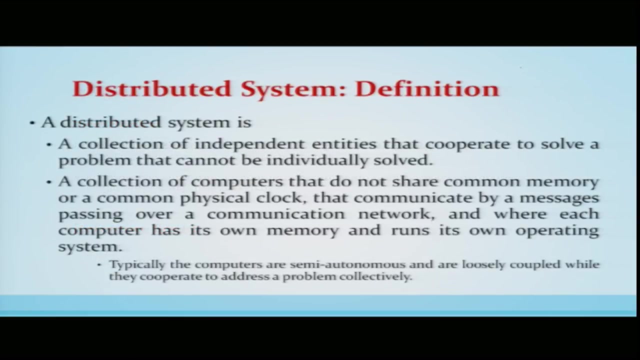 The first will deal about the systems perspective, The first one mentioned here as the authors Shim Kalyani and Singhal. the other text books will deal with the algorithms perspective and that is by Jennifer Welch. We have the reference book also that is distributed algorithms by Nancy Lynch. 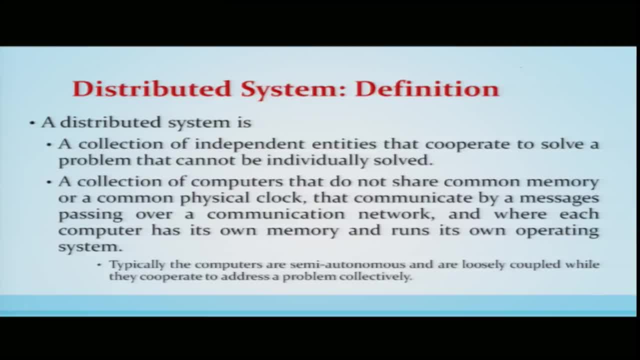 Let us begin with the definition of a distributed system. Distributed system is a collectible system. It is a collection of independent entities that cooperate to solve a problem that cannot be solved individually. So, basically, it is nothing but a collection of computers. thus this particular collection. 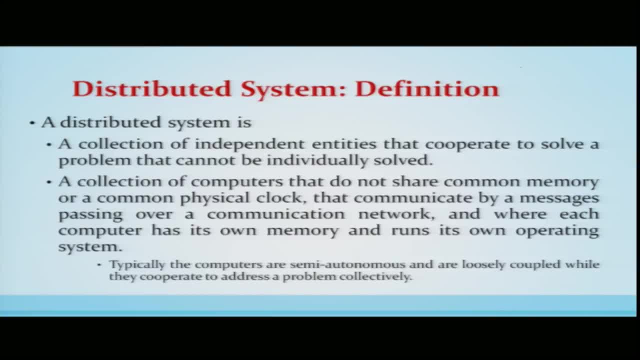 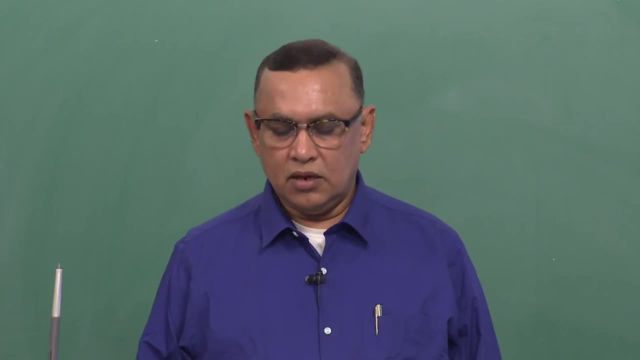 do not share a common memory or do not have a common physical clock, and the only way they can communicate is through the message passing, and for that they require a communication network. The computers used here in distributed systems are semi-autonomous and they are loosely coupled. 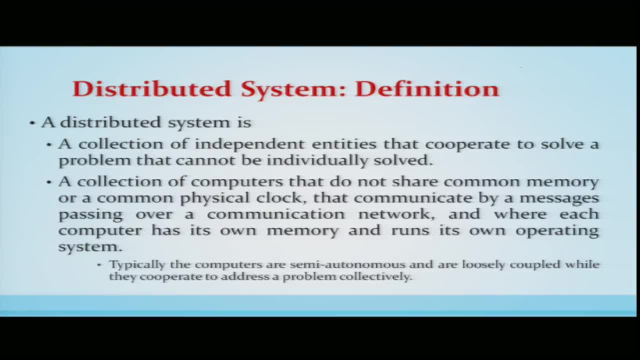 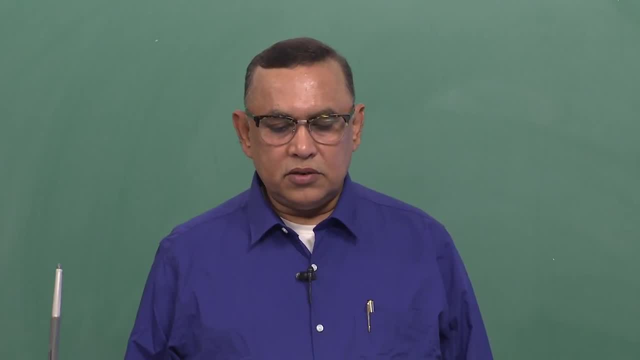 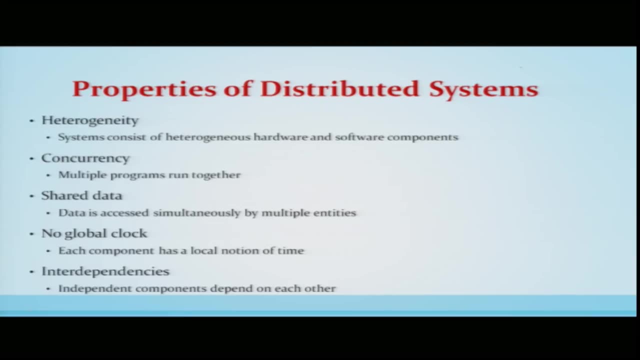 while they cooperate to address the problem collectively. So before we understand in more detail about the distributed system, let us have some properties of a distributed system to keep in your mind at this point of time. So heterogeneity is one of the properties, because here the system comprises of different 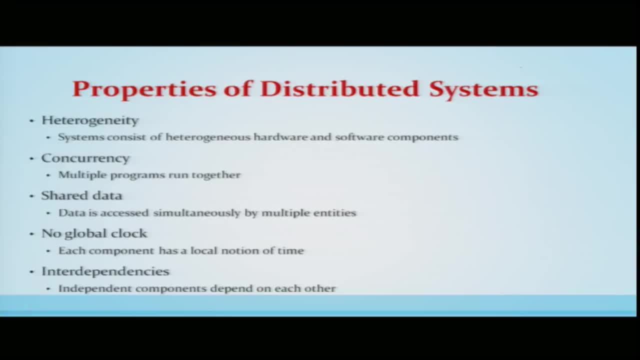 computers, autonomous computers, and they may be heterogeneous, having heterogeneous hardware and software components. The concurrency is another property of a distributed system. Shared data is also another property of a distributed system. So no, global clock is also one of the important properties, and interdependencies are there. 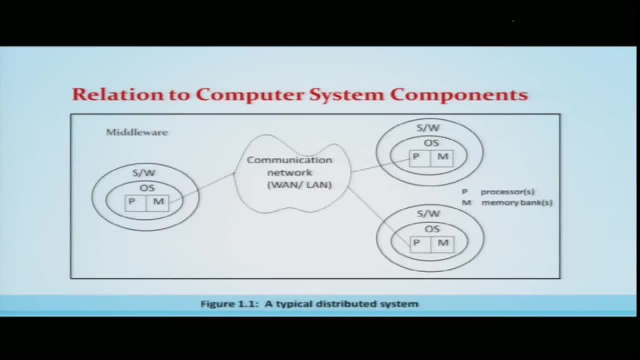 The interdependent components depend on each other. Now to understand the distributed system From the system perspective, let us see this particular figure diagram. In this particular diagram you can see the computers, or autonomous computers, represented as processor memory, with the operating system and, basically, the communication protocol stack. 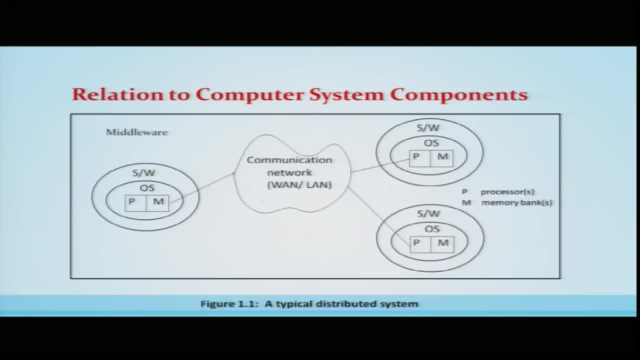 and this particular, these different computers. they can communicate through the network, that is the communication network. Now, as far as the software is concerned Which will build up distributed system, This particular software is called basically the middleware, and the part of these middleware is basically the software which runs on each computer. okay, 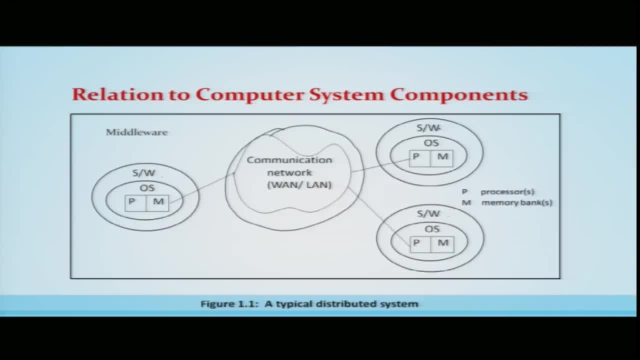 They are called softwares, They are written as the software components. So basically this particular distributed system software will basically use the existing computers, their operating system and underlying computer network and they run the part of the middleware And together this will form a distributed system. 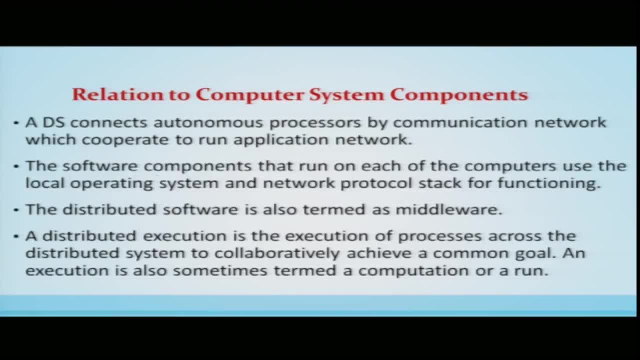 So middleware will bind the distributed system. So again further explain. the distributed system connects autonomous processors by communication network and the software component that run on each of the computers use the local operating system and network protocol stack. The distributed software is termed as middleware. The distributed execution is the execution of the processes across the distributed system. 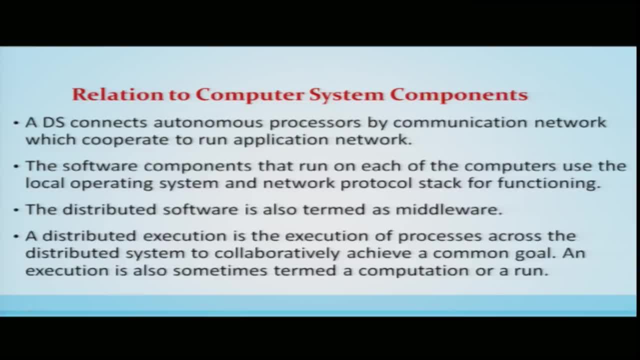 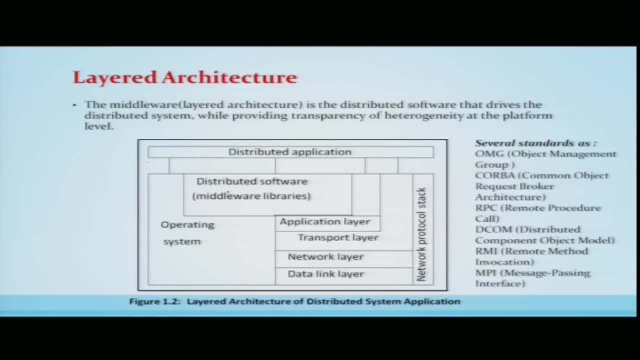 To collectively achieve a common goal. The execution is also sometimes termed as the computation or error in a distributed system. Furthermore, the distributed software, which is also called a middleware, is designed in a layered architecture to simplify the complexity of the distributed software And this particular middleware, or the distributed software that drives the distributed system. 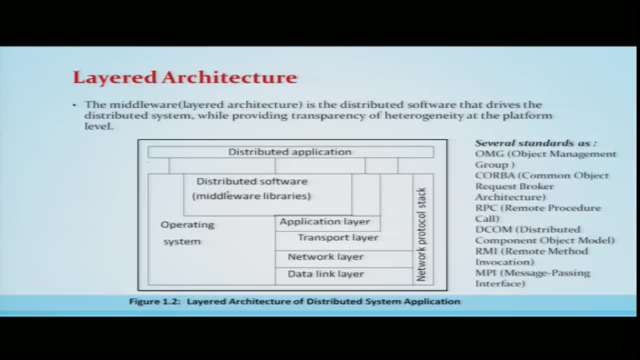 It also provides the concurrency of heterogeneity at the platform level. So in the diagram you can see the distributed application mentioned over here. So this particular distributed application will use the distributed software, which is a middleware. Middleware runs on the operating system of each collection of computers and also it will 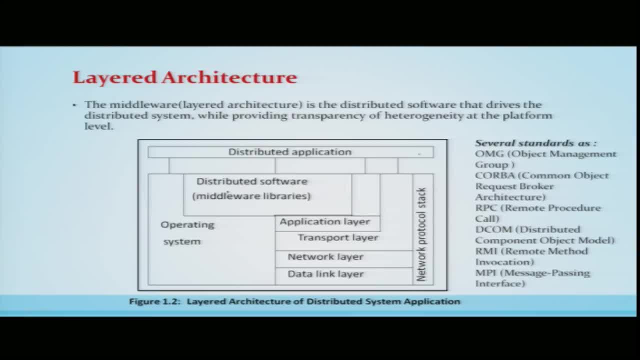 use the underlying network protocol stack for the communication and there are several standards also evolved over it, evolved over a time for this particular middleware, application, middleware for the distributed software development, that is, OMG, CORBA, RPC, DCOM, RMI, MPI and so on. 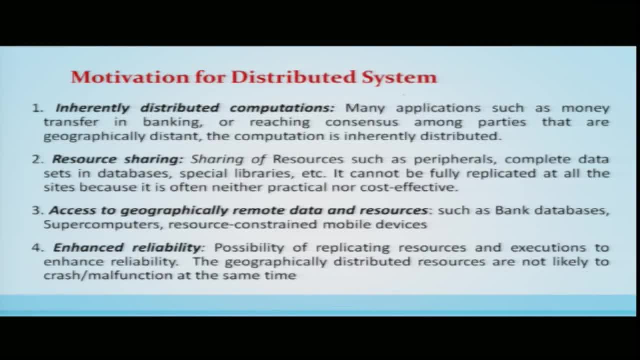 So that was the overview of the distributed system from the system perspective. Now we are going to touch upon the motivation of the distributed system. So inherently distributed computation, that is, many applications such as money transfer in the banking, are reaching a consensus among the parties that are geographically distant. 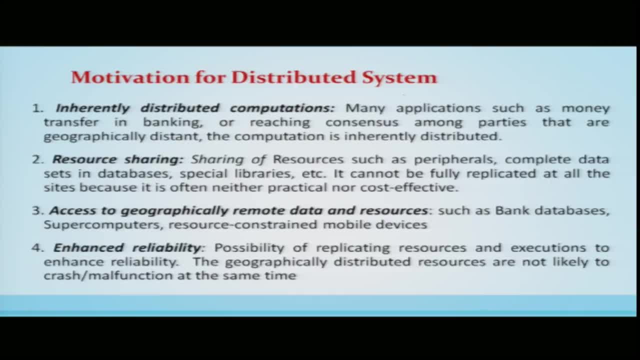 the computation is inherently distributed. So for that the model, that is distributed system, is required for that computation, that is, the applications which are inherently distributed. Then next is the motivation called distribution, Resource sharing, the sharing of the resources, such as peripherals and complete data set. 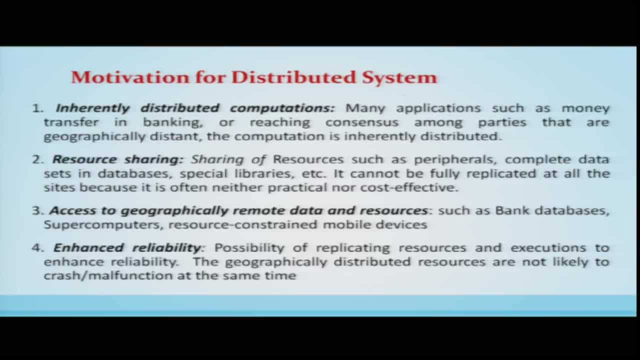 and so on and so forth is basically the motivation behind this building of distributed system. Another motivation is to access the geographically remote data and resources, such as bank database, super computer and so on. Reliability, enhanced reliability, possibility of replicating the 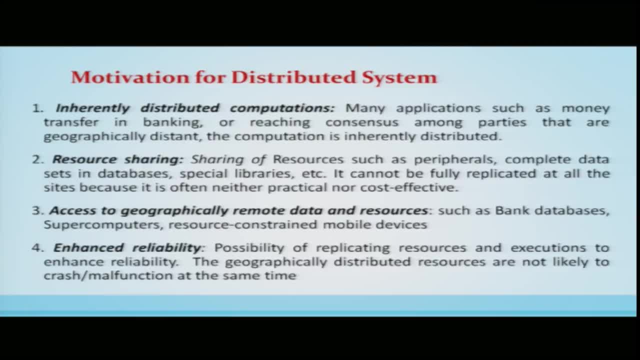 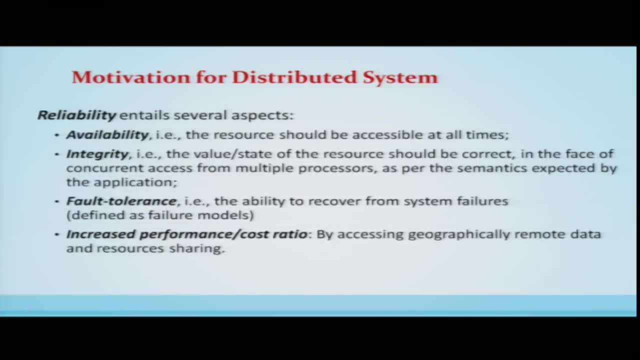 resources and execution to enhance the reliability. Geographically distributed resources are not likely to crash at the same time. That is the motivation of building the distributed system for that. So reliability entails several aspects in that case. So these are basically the availability- The resources should be accessible at all the times. Integrity, the value or oblique. 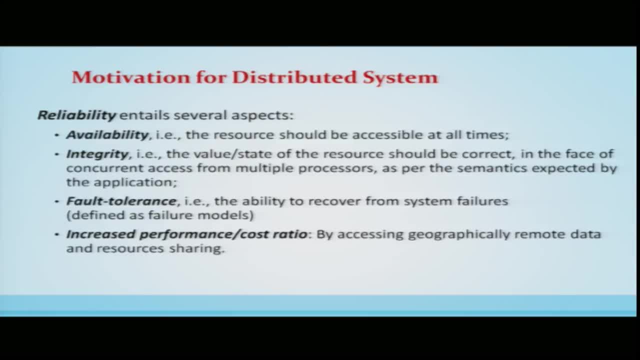 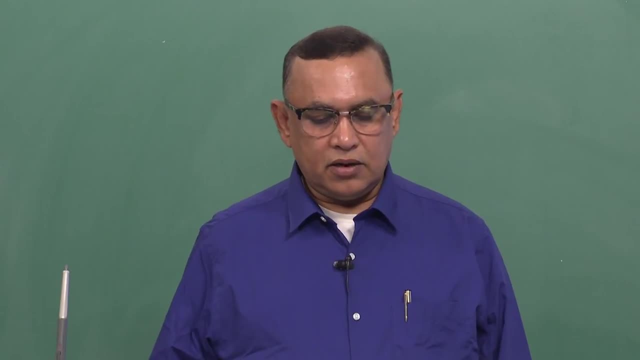 the state of the resource should be correct in the face of concurrent access And fault tolerance. the ability to recover from system failures, Increased performance of the system, oblique cost ratio by accessing geographically remote data and resource sharing. So these are basically the reliability will entail these aspects. So basically other advantages of distributed system is scalability. adding more processor to the communication network does not pose a bottleneck to the communication network. Then the next advantage is modularity and incremental expandability. So here the processor, the heterogeneous processor, can be added without any bottleneck problems. 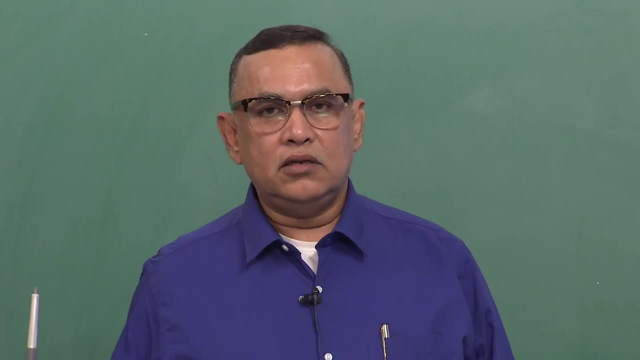 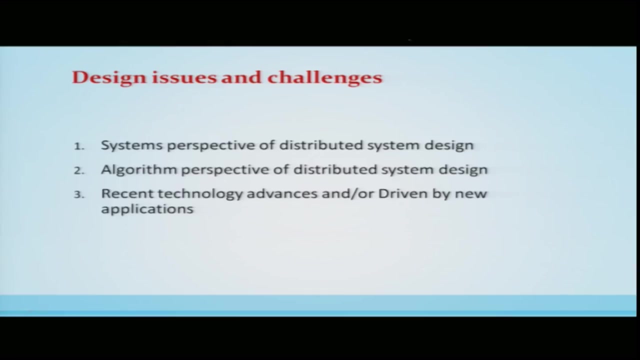 Now we are going to discuss the design issues and challenges in the distributed system design. So from system perspective of a distributed system design, we are going to see what are the intricacies and we have to understand the theoretical basis for this design. Another thing is algorithmic perspective of a distributed system design. The next design issues and 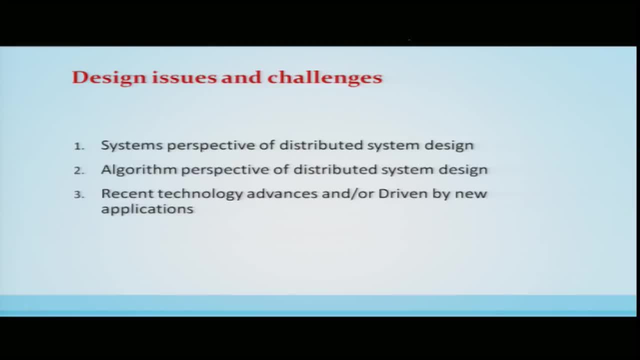 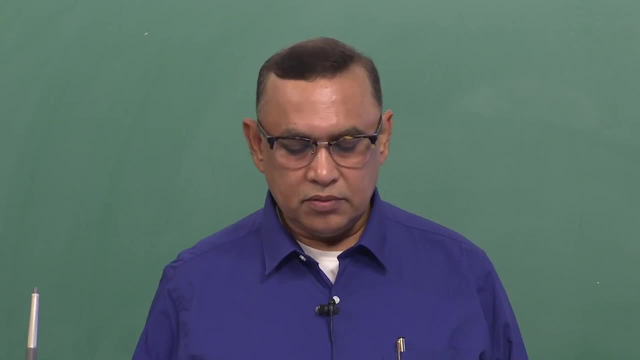 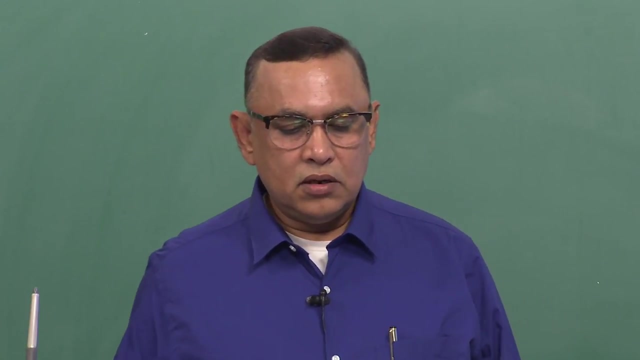 challenges is based on the recent technology advances and also driven by the new applications and which will basically be the motivation or be the design issues and also becoming a challenges in evolving the distributed systems. So, firstly, we are going to look upon the design challenges from system perspective of distributed 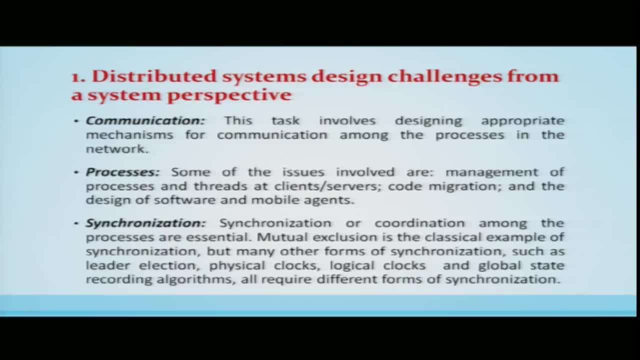 systems. First of all, the components which are involved here in the system's perspective are the communications, that is, the communication network where the processors can basically communicate with each other, through which processors can communicate Processes. some of the issues involved are the management of the processes and the threats. 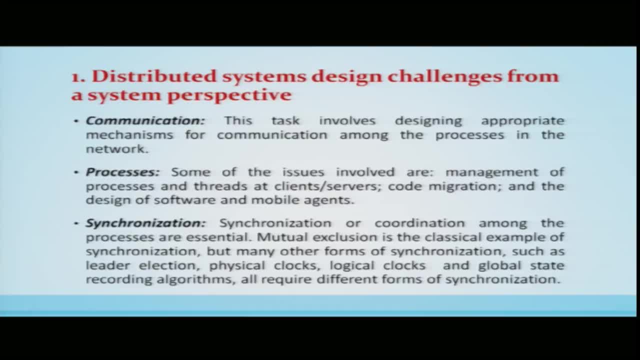 At the client server, code migration, design of software, mobile agents. synchronization is the most important part. Synchronization, or the coordination among the processes, are essential. virtual exclusion is an example of a synchronization, but many other forms of synchronization, such as leader election, physical clocks, logical clocks, global state recording algorithms. 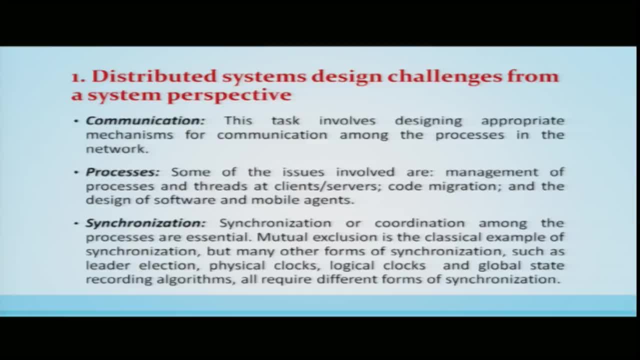 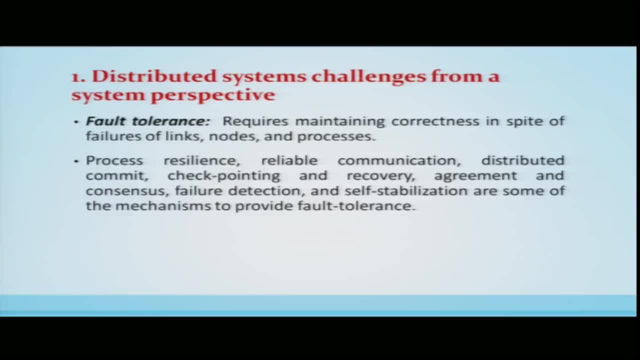 all require different form of synchronization that we are going to cover up in this part of the course in more details. Now, another system level challenge is the fault tolerance. So this fault tolerance: it requires maintaining correctness in spite of the failures of links, nodes and processes. 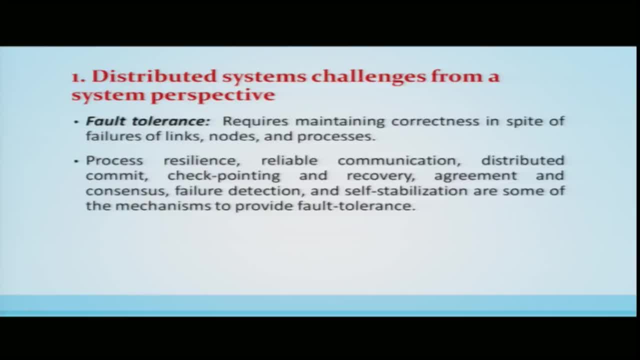 So this particular fault tolerance is basically achieved using the process: resilience, reliable communication, distributed commit, checkpointing and recovery, agreement and consensus, failure detection, self stabilization. These are some of the techniques which we are going to cover up when we discuss the. 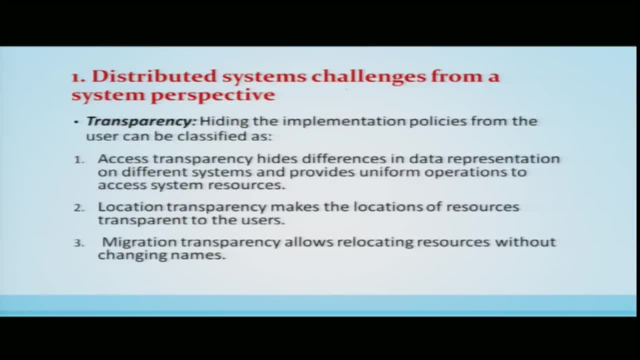 design from system perspective. Another system perspective design Angle or aspect is transparency. So transparency is to hide the implementation policies from the user, and this can be a different kind of transparencies. The first one is called access transparency, when it hides the differences in the data. 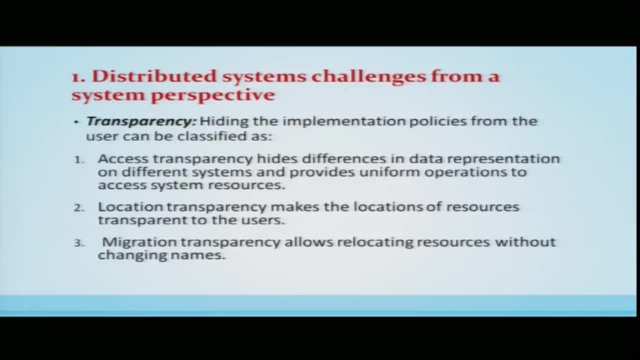 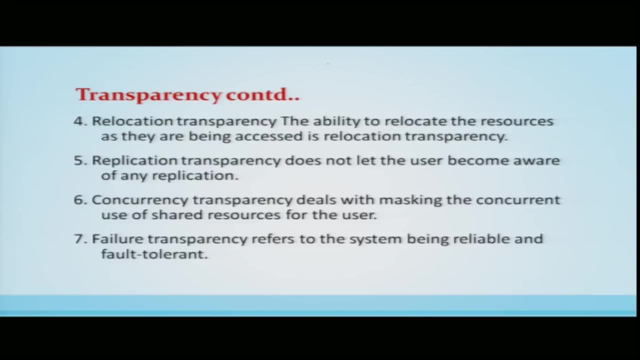 representation on different systems and location transparency when it makes the transparency of the location of the resources and migration transparency allows the relocating resources without changing Relocation transparency- the ability to relocate the resources as they are being accessed- is relocation transparent. Replication transparent does not let the user become aware of any replication. 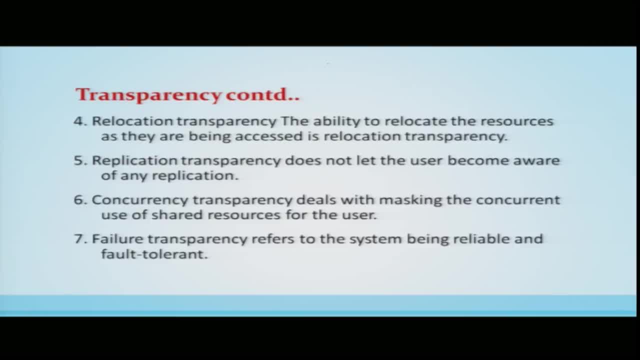 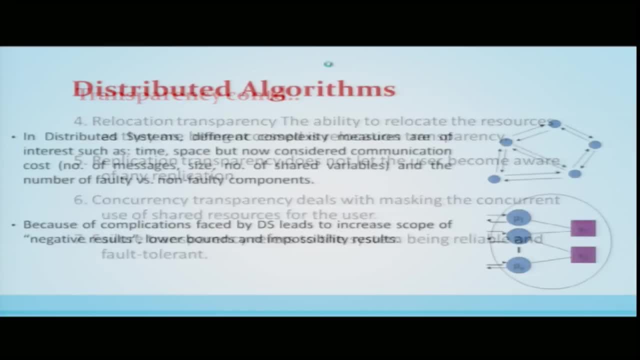 Concurrency. transparent deal with masking the concurrent use of shared resources. for the user, Failure transparency refers to the system being reliable and fault tolerant. it is not known to the user at this at any point of time. Now, that was the distribution, That was the distributed system from system perspective. 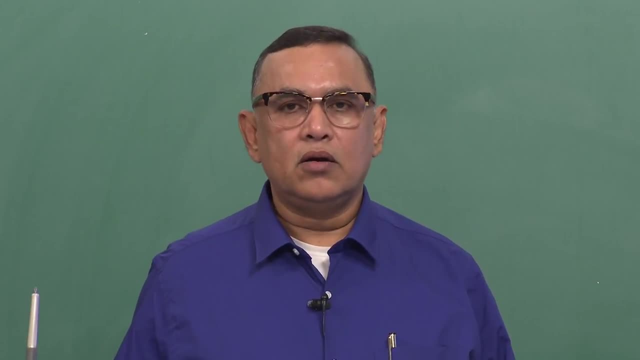 Now we are going to touch upon another important component of this particular distributed system, distributed computing system that is called distributed algorithms. So the algorithms are to be evolved. So we are going to cover up the fundamental algorithms which will be the building, basic building block of developing the distributed applications. 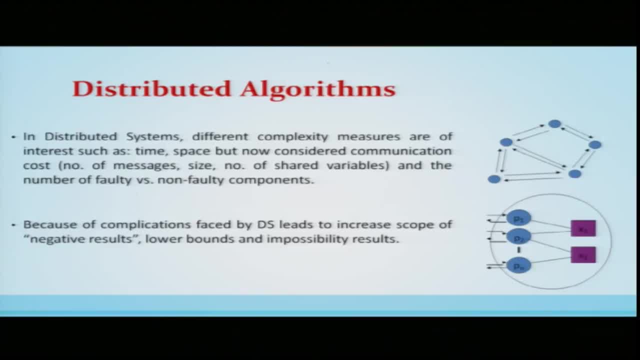 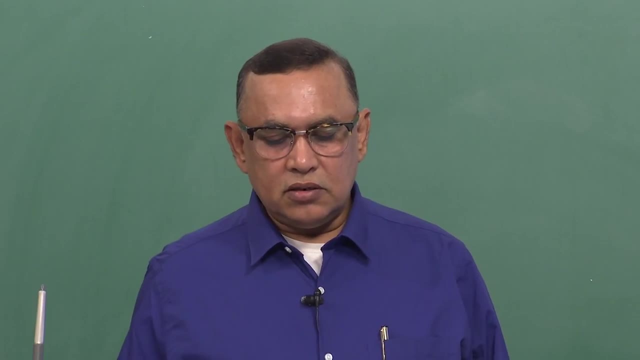 So in distributed applications, Distributed systems, Different, Different complexity measures are of interest, such as the time and space. They were used in the classical or the sequential algorithms as well, but now communication is also evolved, So communication cost is one of the complexity measure. 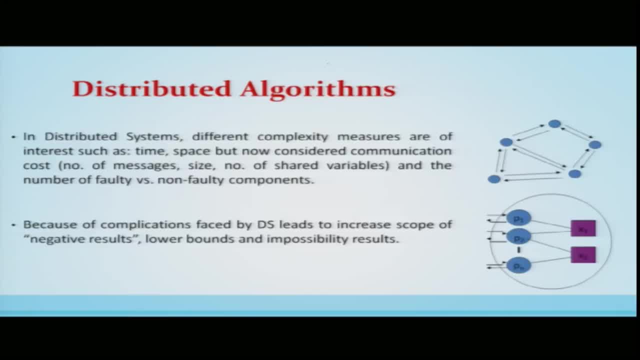 So communication cost includes the number of messages, size of the message and number of shared variables, And also another component, Component, Component which will be used in the complexity is called basically the number of faulty versus non-faulty components. Now, because of the complications faced by distributed system, they lead to the increased. 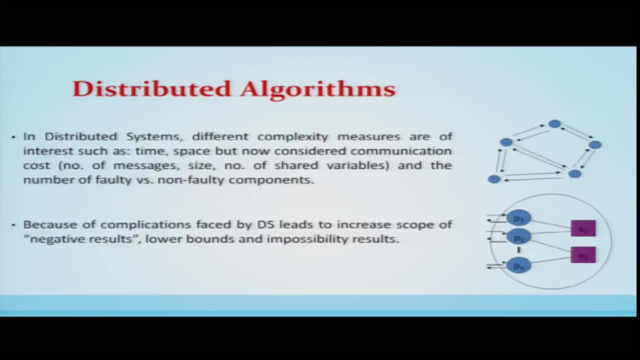 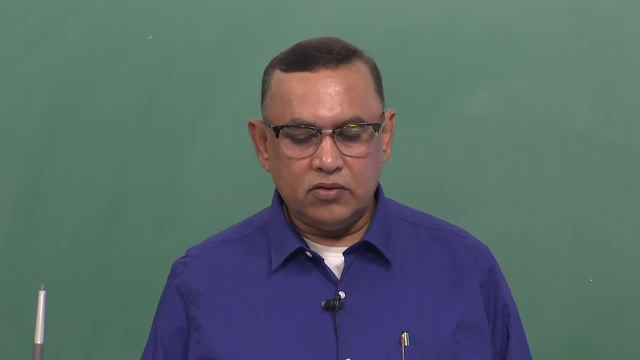 scope of negative results, lower bounds and impossibility results. So all these things will be covered up in a form of a in the distributed algorithm design, and thus we will discuss more these particular distributed algorithms later. Thank you, Thank you, Thank you. 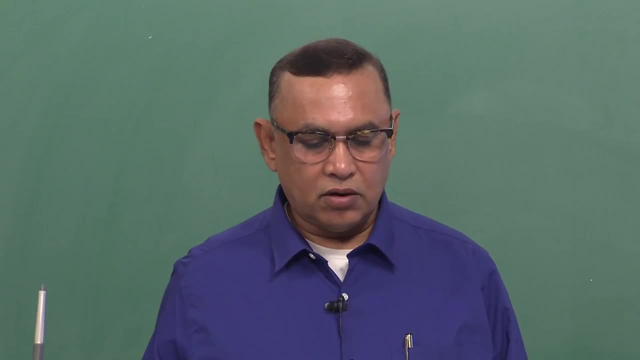 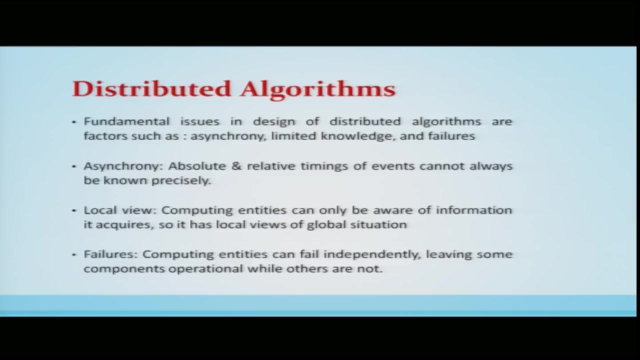 So let us focus in the details of. So the fundamental issues in the design of distributed algorithms are the following three factors: The Asynchrony. So Asynchrony, limited knowledge and failures. There are three different important fundamental design issues in the algorithm distributed. 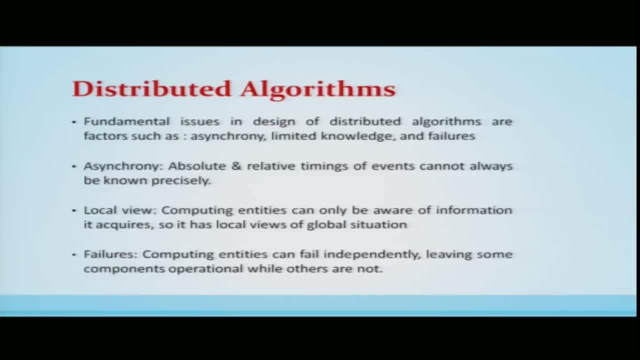 algorithm Asynchrony is basically absolute and relative timing of the events cannot be known precisely, So in this particular setting, how the algorithms are to be evolved and developed- Local view that is, the computing entities can only be aware of the information it acquires. 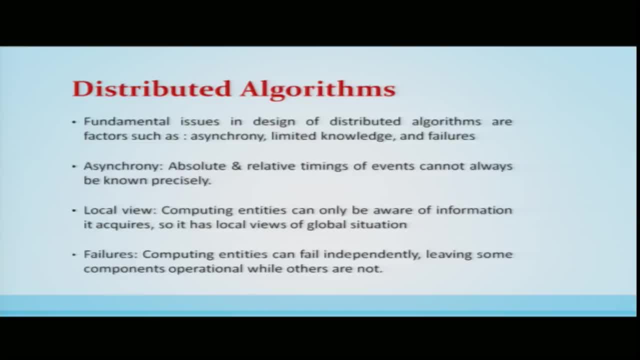 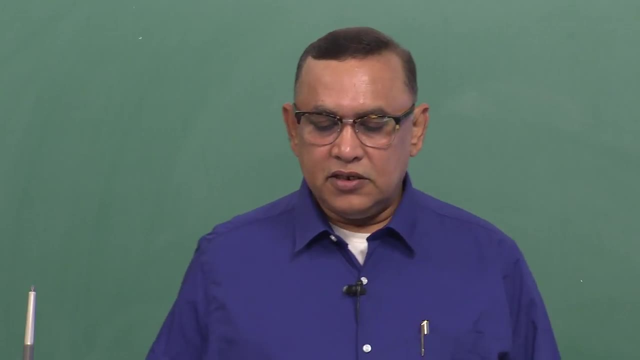 So it has only the local view of a global situation. Third one is the failures. So the computing entities can fail independently, leaving some components operational while others are not. So these three different factors, they add the more complications in design of the distributed 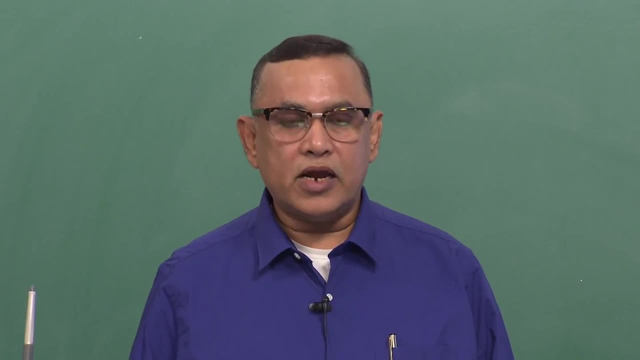 algorithm and becomes a challenging to evolve the distributed algorithm in these particular problem setting. that is, as synchrony That is, we are not knowing the events, when it they are going to occur- Local view. we are not knowing the complete picture of the global situation yet we have 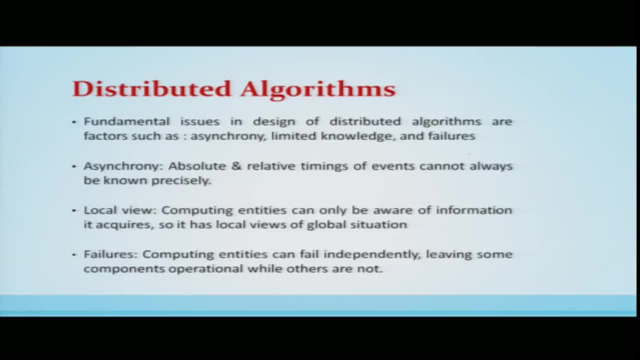 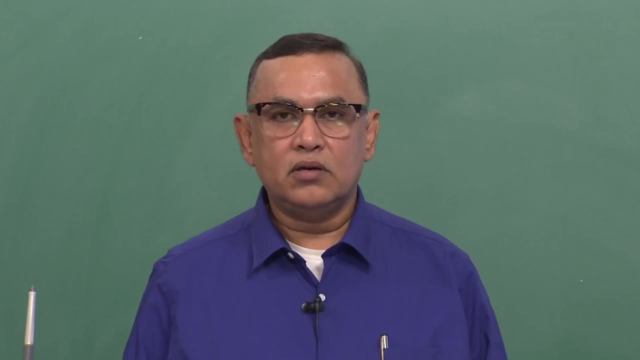 to come up with an algorithm. Failures means the components which are basically in Involved in that distributed systems. they can fail independently and basically it is expected that the applications should basically keep on running in spite of failures. So distributed computing systems studied since 1967, starting with Dijekstra and Lampard. 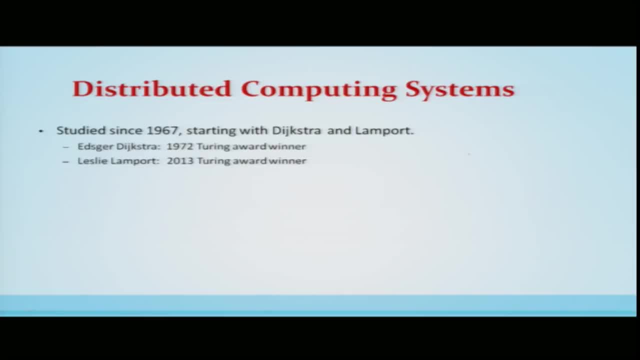 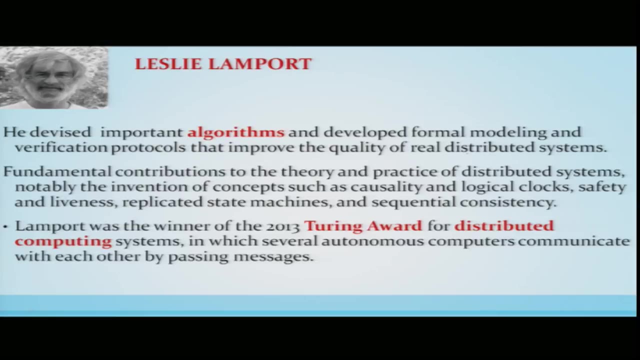 Dijekstra in 1972 got tuning award for the works on the distributed algorithms and distributed systems. Leslie Lampard very recently has got the tuning award for his work on basically the distributed algorithms and systems. Special mention to the Leslie Lampard because most of the works, whatever he has done, we 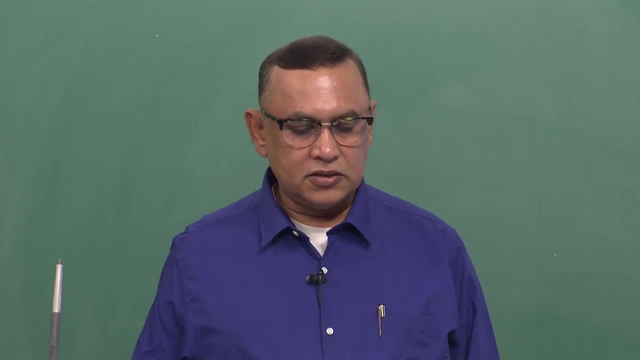 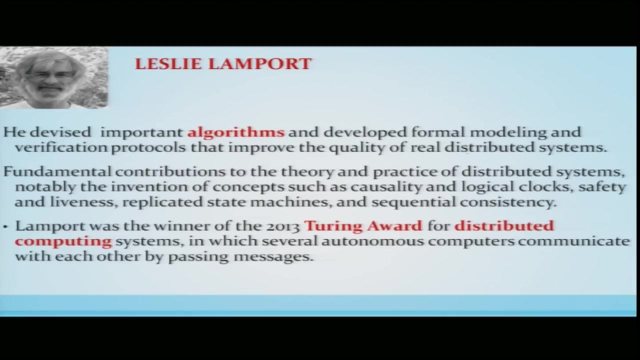 are going to cover up as far as distributed systems fundamentals are concerned. So Leslie Lampard: devised important algorithms, developed formal model verification protocols to improve the quality of real distributed systems. fundamental contribution to the theory and practice, Notably the inventions of the concepts such as causality- look logical, clock safety. 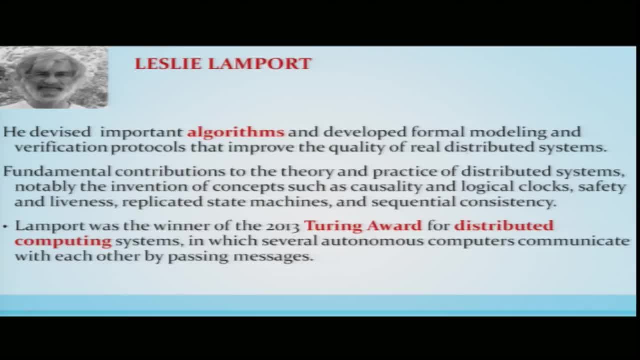 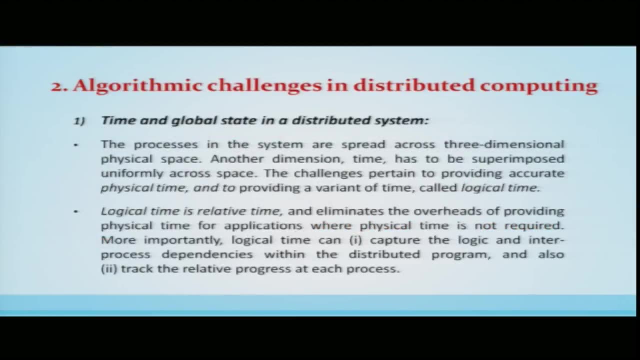 and liveness. replicated state machines, sequential consistency, are some of them. So Lampard was the winner of 2013. that is tuning award for distributed computing. Now algorithmic challenges in the distributed system we are going to touch upon. that is. 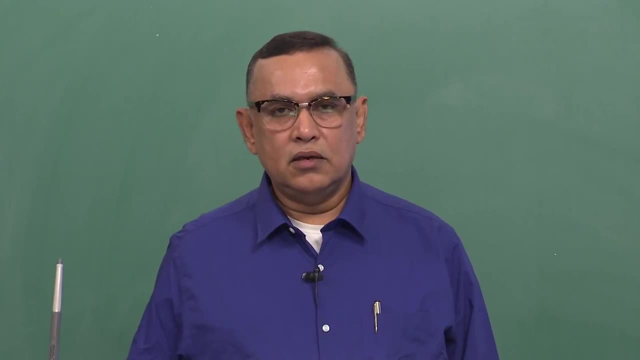 previously. we have seen the distribution, So we are going to touch upon that. So we have seen the distribution, So we are going to touch upon that, So we want to touch upon that. So the desing challenges from system perspective. 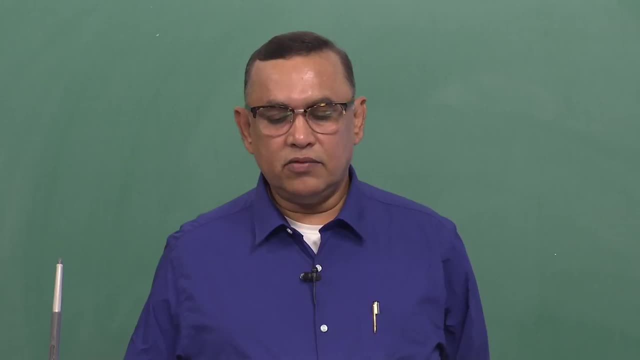 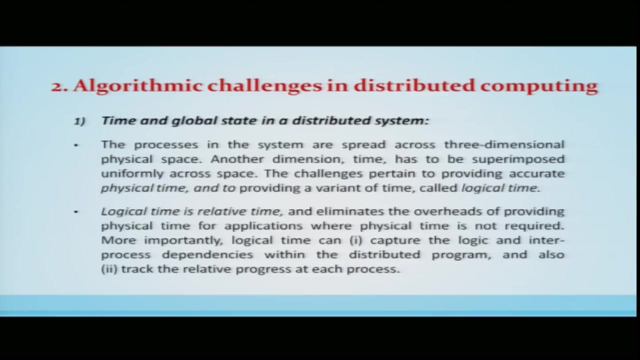 Now we have to see the algorithmic challenges: developing the distributed systems, Designing the distributed systems. So time and global state in a distributed system. So this is the important challenge. Let us see what this is. The processes in the system are spread across three dimension of physical space. 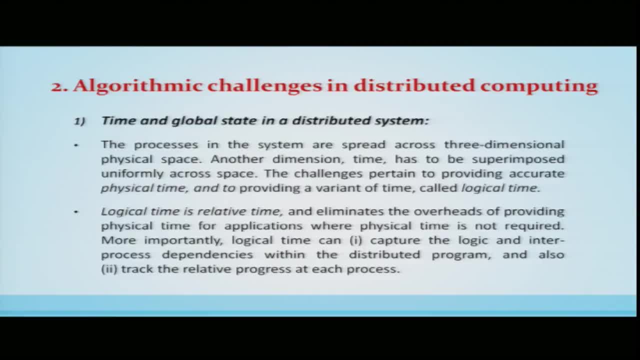 Another dimension is the time. Time has to be superimposed uniformly across the space. The challenges pertain to providing accurate physical time, because there is no common clock, and to provide a variant of a time that is called a logical time. So logical time is a relative time and eliminates the overhead of providing the 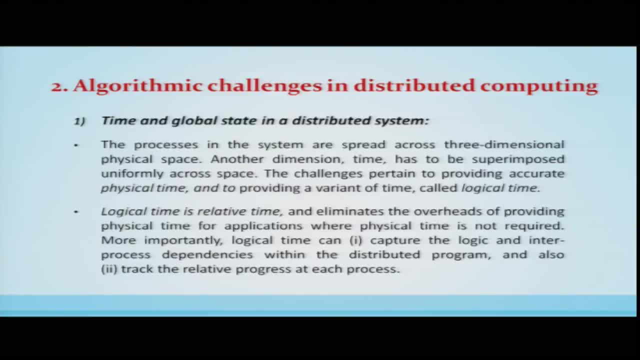 physical time for the different applications and basically the logical time basically can capture the logic and the inter-process dependencies within the distributed program and also track the relative progress at each process. So instead of physical, having a common physical clock or basically implementation of a common physical clock, here we are going to see the 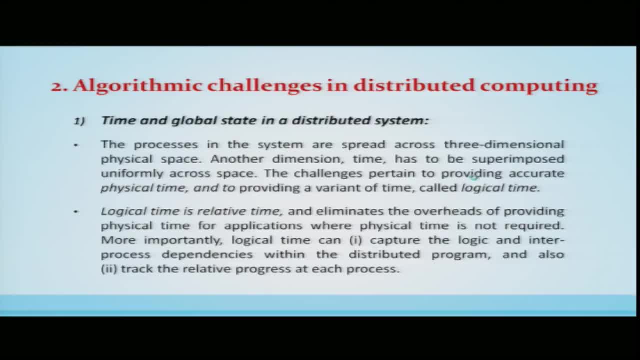 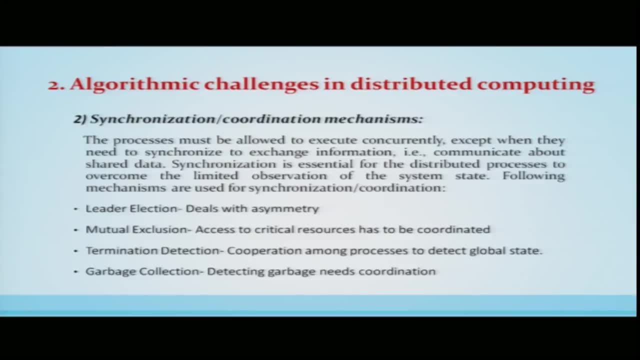 how the logical clock can solve, without having the physical clock, these particular problems. The other problem, other algorithmic challenge, is the synchronization coordination mechanisms. So the processes must be allowed to execute concurrently, So concurrently accept when they need to synchronize to exchange the information. that 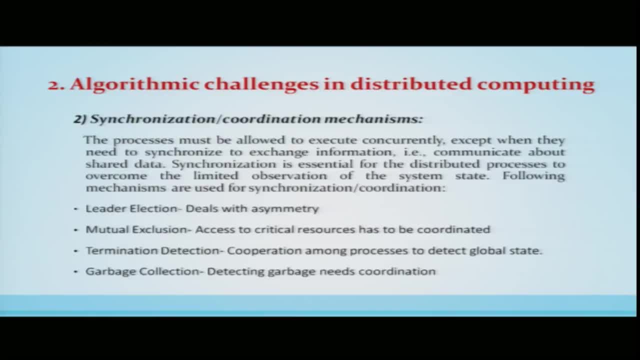 is communicate about the shared data. So synchronization is essential for the distributed processes to overcome the limited observation of the system state. The following mechanisms are used for the synchronization and the coordination: First of all, leader election deals with the asymmetry of a process and then mutual exclusion. 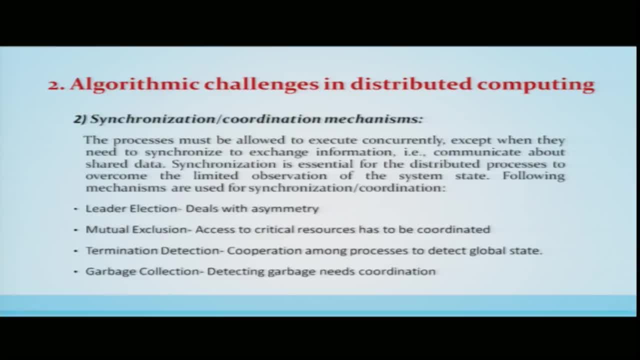 Access to the critical resources has to be coordinated through. that is done through mutual exclusion. Then termination detection, that is cooperation among the processes. they will basically able to detect the required state, the required global state. that is called termination state and that is called termination detection in a distributed system. The next important 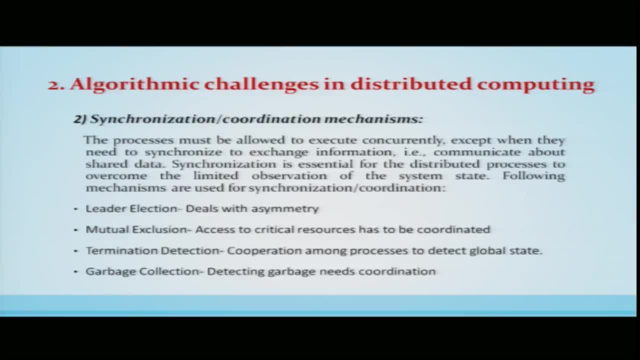 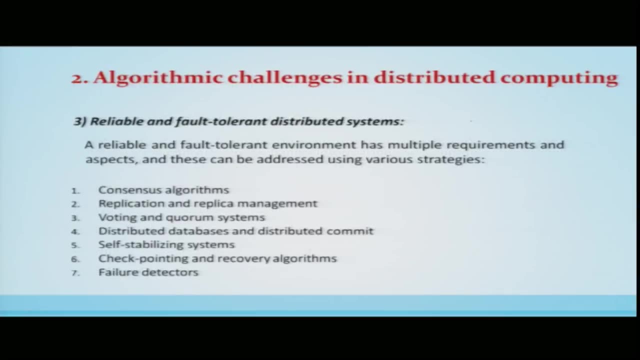 that means thing is called garbage collection. detecting the garbage requires another, the coordination. So these are basically the synchronization and coordination mechanisms which will basically be the used up in designing the distributed applications. Another thing is another important notion is the reliable and the fault tolerant distributed 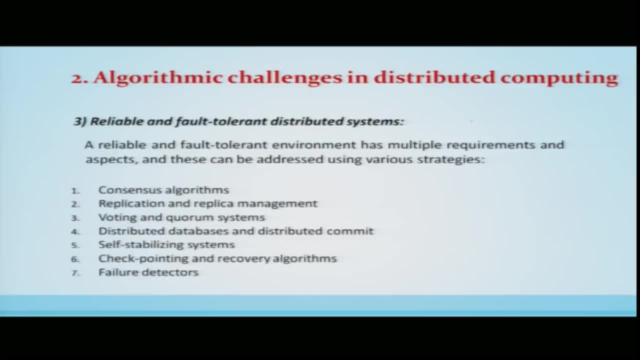 system, So reliable and fault tolerant environment, has multiple requirement aspect and these can be addressed by the various strategies which we are going to cover up in this part of the course. The first one is called consensus algorithm. Second is replication and the replica management, voting and quorum systems, distributed databases and distributed commit self stabilization. 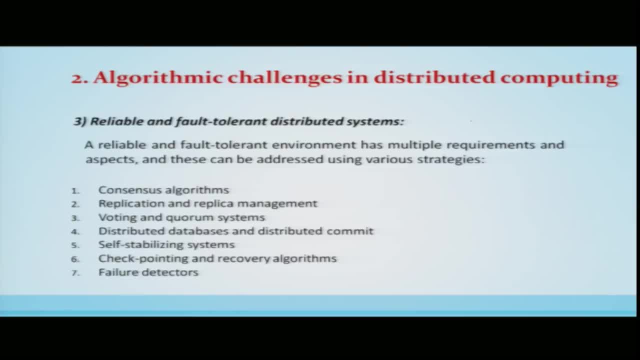 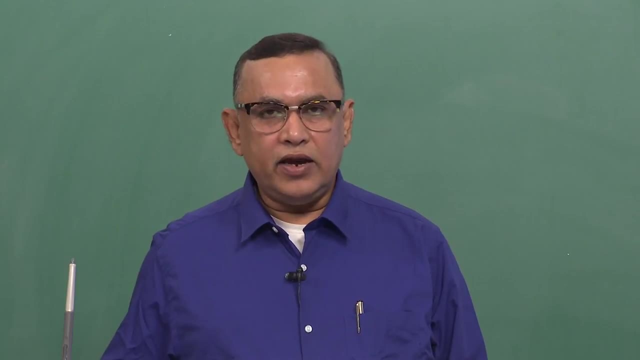 system and check pointing and recovery algorithm and failure detectors. So these together, these strategies, will be able to provide the fault tolerance, that is, if the component, like nodes, links, are failing, yet how the distributed application can basically work on without any disruptions. and that is the main requirement of the materials of a 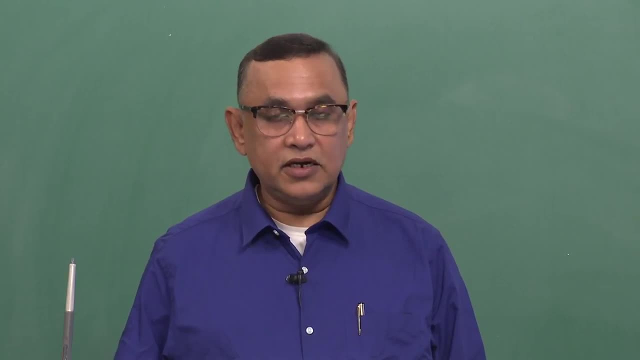 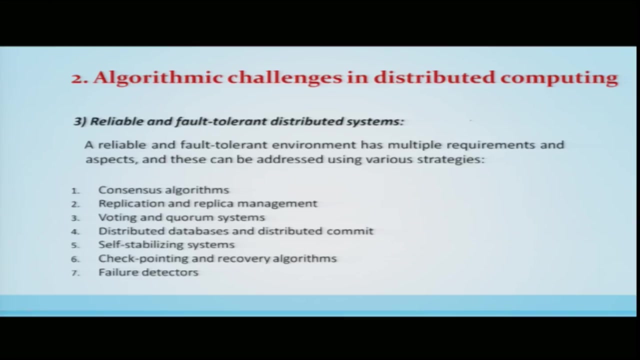 distributed system to have reliablestream in the distributed system. So, basically, if the processors or the algorithms which are required, or consensus algorithm, because n the failures, Etc克 Democrations. 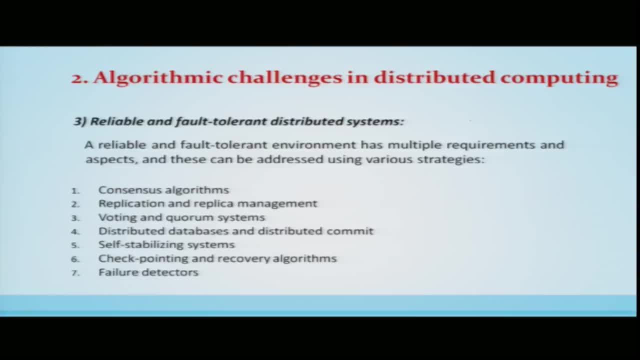 So the remaining non-faulty processors. they have to basically come up with their consensus on the values, and the applications are continuing to run. Another thing is called replica and replica management, because if replicas of that data is available, then the application can run without the problem of failures. 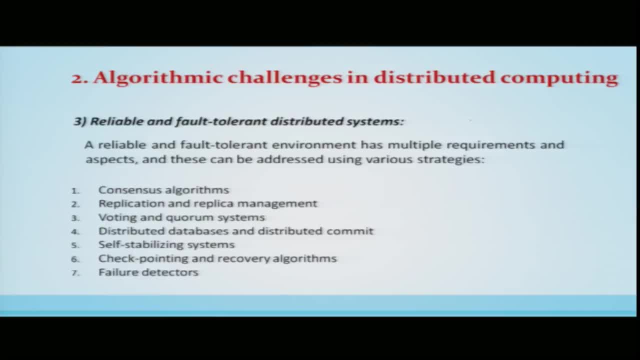 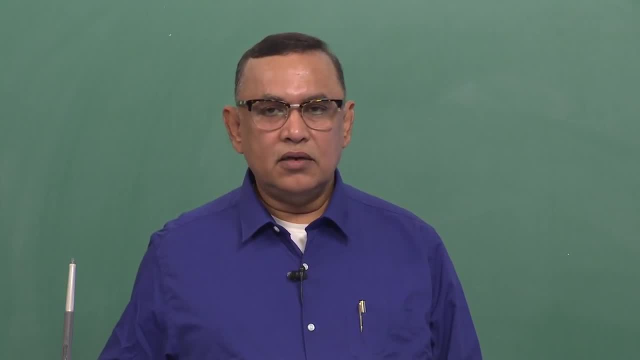 Then voting and the quorum is also a important criteria. for example, when some of the systems are, when some of the important system is failed, then basically the among the remaining, they have to evolve through the voting and quorum mechanism to basically run those applications. 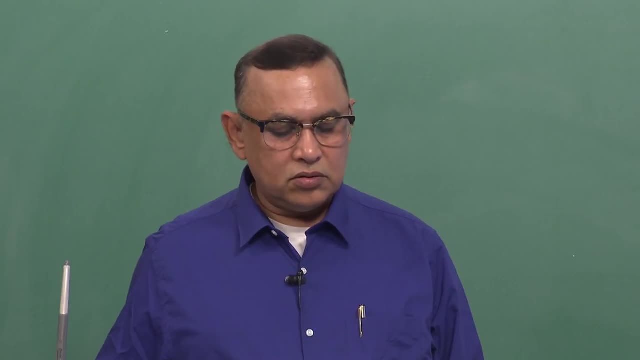 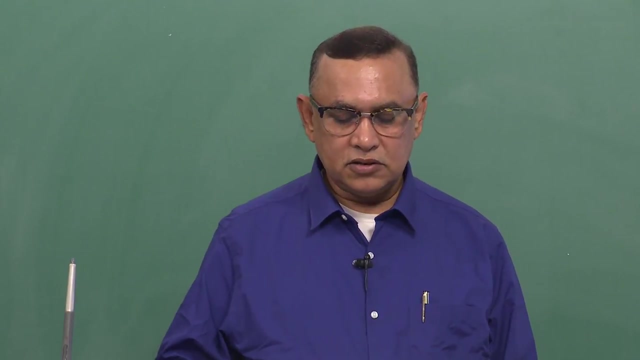 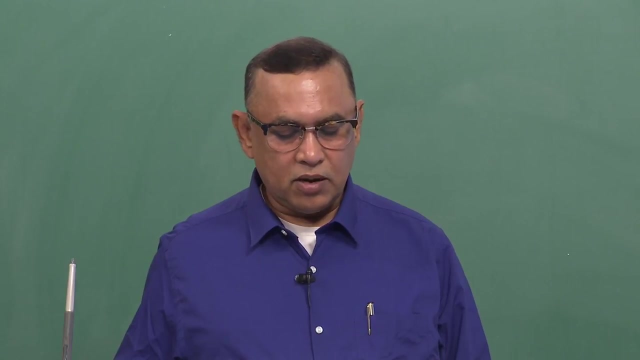 And distributed databases and distributed commit is also basically one of the important applications where they have to decide among discussion with each other. They have among the synchronization to see whether the commit which is taking place has to be done Or has to be aborted by taking the decisions. 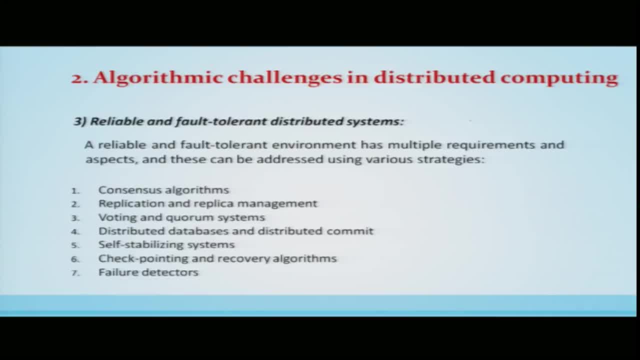 Then. self-stabilization system means, if the components are failing, then how the system evolves and how much time it takes to stabilize itself. So that is self-stabilization systems that we are going to also cover up briefly in this part of the course. 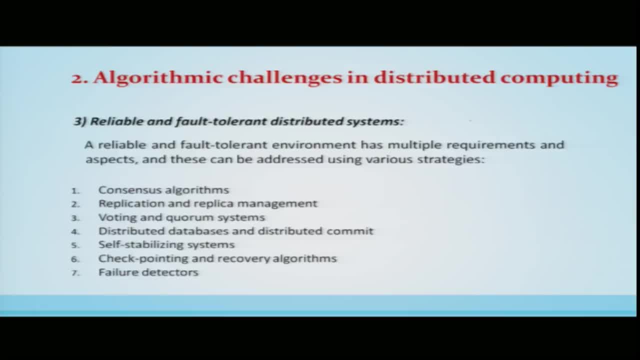 Checkpointing and recovery system are very important as far as the fault tolerant is concerned. Fault tolerant means if there is a failure, How basically the operations which are done has to be basically with a minimal loss, has to basically resume their operations. So checkpointing and rollback recovery algorithms we are going to cover up in this part of the 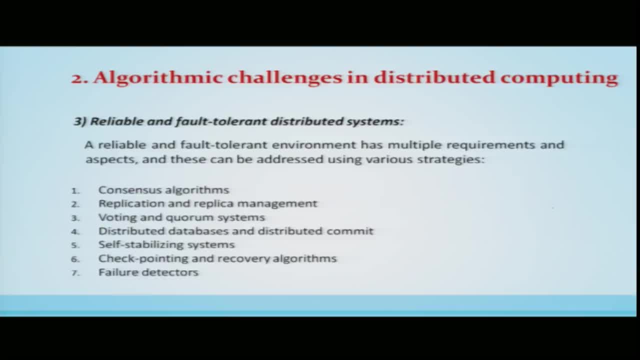 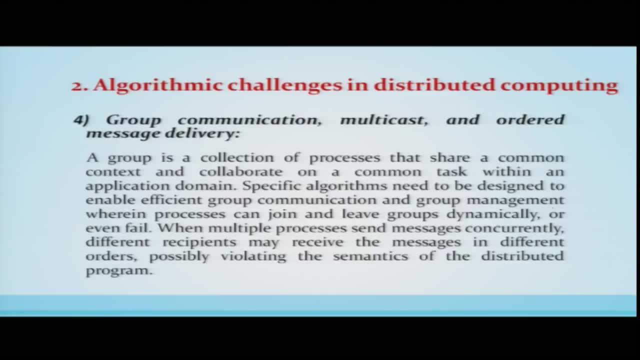 course, Then failure detectors are also very important if how to detect that the nodes or the links are basically not working on a field. Another important algorithmic challenges is basically forming the group communication, multicast and ordered message delivery. So there are some applications where the group communication is required. 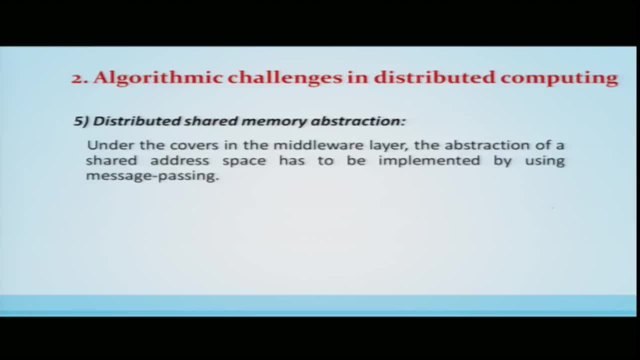 So basically, this paradigm is also useful for them to develop the application Distributed shared memory abstractions. now the middleware is the software, is the distributed system. software will basically use this particular, this one abstraction called distributed shared memory, Although it is not having a common memory. but distributed shared memory is realizable. 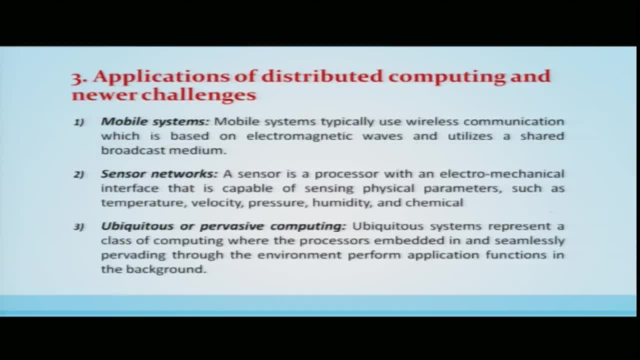 using the message passing systems. So that is what we are going to cover, That we are going to see Now the applications of a distributed computing systems and basically the newer challenges. Mobile systems: mobile systems typically use the wireless communication which is based 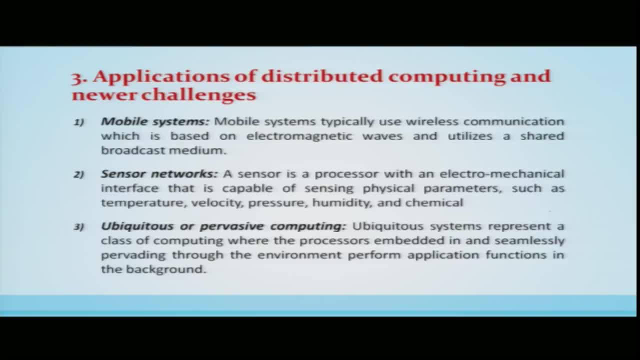 on electromagnetic waves and utilizes a shared broadcast medium. So mobile system is one of the application of a distributed computing application where different elements are involved to come up with this particular service and that is called a mobile service And that is an application of a distributed computing. 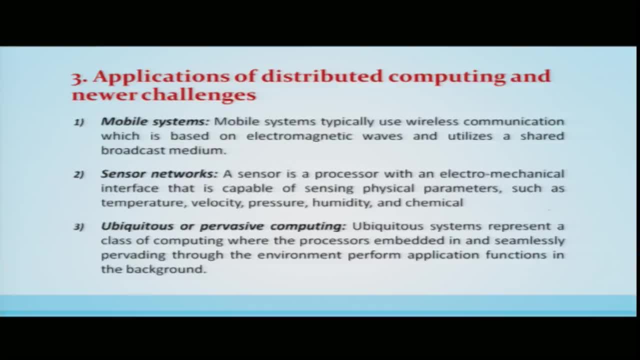 Sensor network is another application. Sensor is a processor equipped with an electromechanical interface and that is capable of sensing physical parameters such as temperature, velocity, pressure, humidity and chemical. So this particular kind of nodes, called a sensor node, if basically deployed to basically. 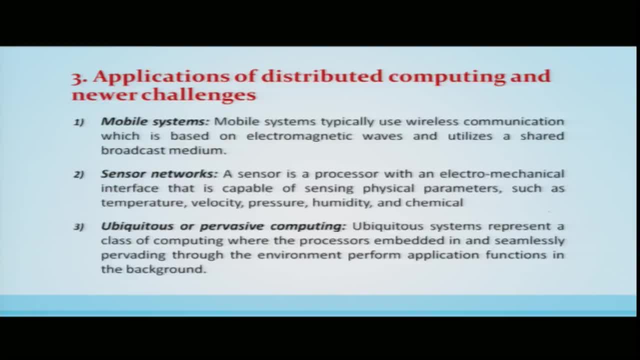 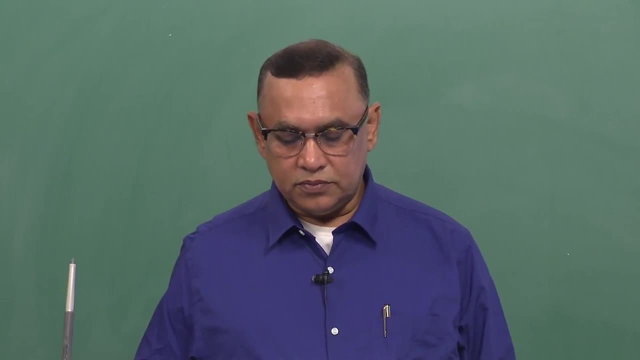 monitor the cyber physical. So we will make a cyber physical system to monitor any physical activity or event, For example to monitor the weather, it is having a volcano eruption or any other situation. So it is having a lot of use in cyber physical system and it is a kind of large scale distributed. 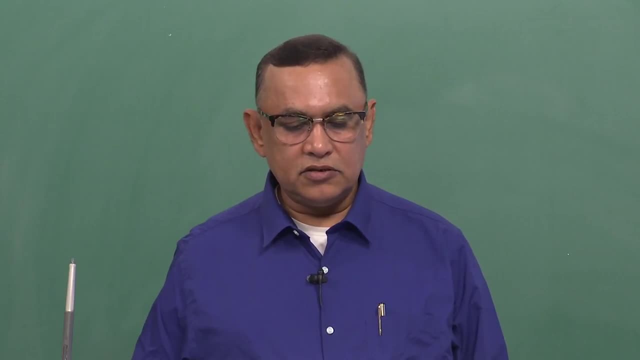 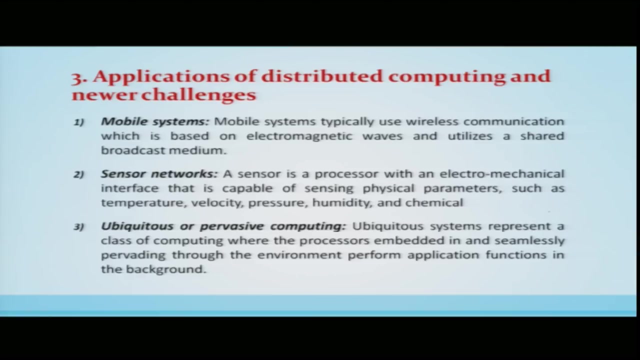 system that we. that is basically using the principles of a distributed systems. Another application here is called UBS, UBS, So ubiquitous or a pervasive computing. ubiquitous systems represent the class of computing where the processors embedded in seamlessly providing through the environment perform the applications. 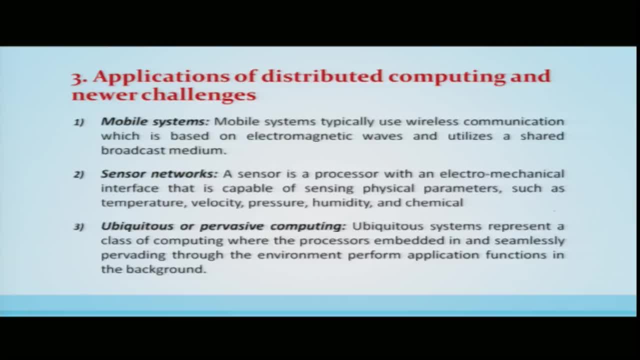 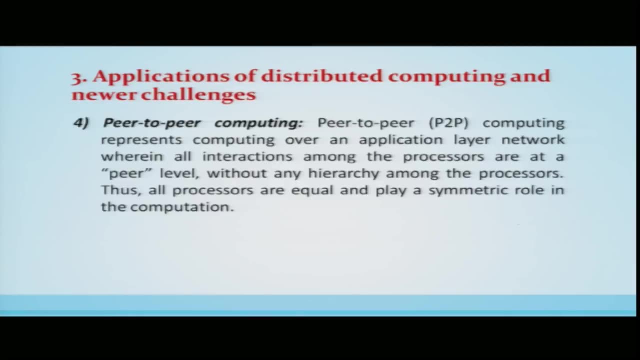 functions in the background. Examples are the smart environment. smart environment or a smart buildings, smart cities. all are examples of a ubiquitous and pervasive computing. Another application is basically called peer-to-peer. Okay, So peer-to-peer represents the computing over the, over the application network, where 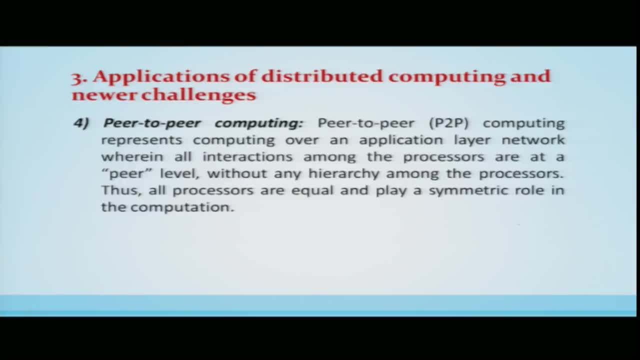 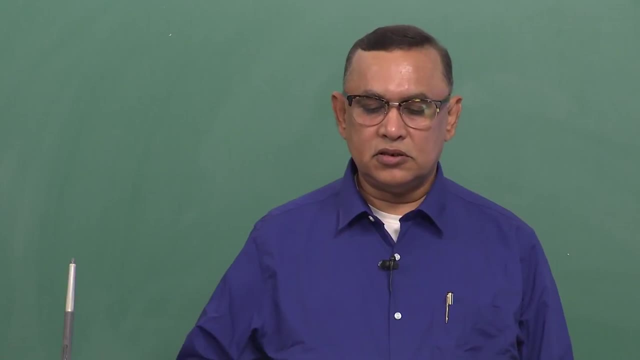 all interactions among the processors are at the peer levels, without any hierarchy among the processors. Thus all processes are equal and play a symmetrical role in the computation. So peer-to-peer network systems are used in providing the resources and the services. Peer-to-peer networking is now basically very challenging. 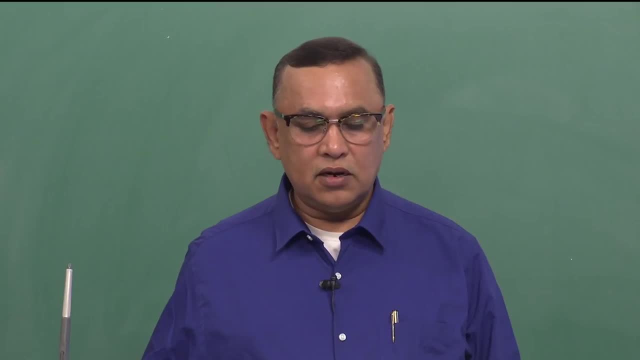 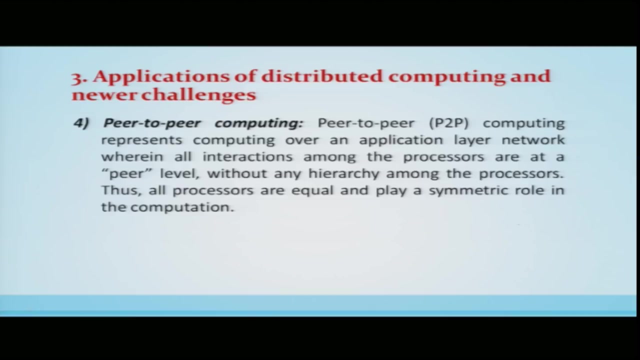 As far as peer-to-peer networking is concerned, Okay, So it is very challenging. as far as developing distributed applications are concerned, Technically also it is quite difficult and but the simpler model, like client-server paradigm, which is not purely peer-to-peer, it is not purely distributed. 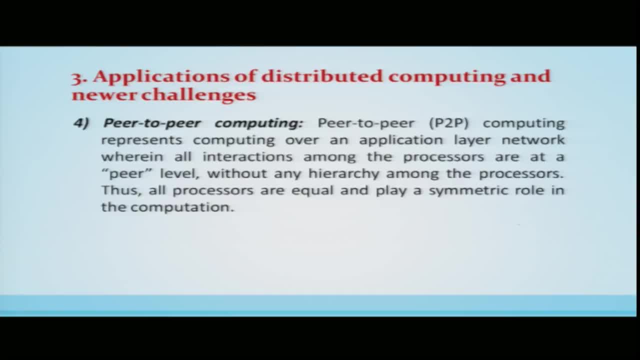 This is used by the different applications because industry feels comfortable with client-server model. Peer-to-peer computing models for different applications are evolving over a period of time. The recent application which is added is called Bitcoin, and Bitcoin is based on peer-to-peer distributed computing design. 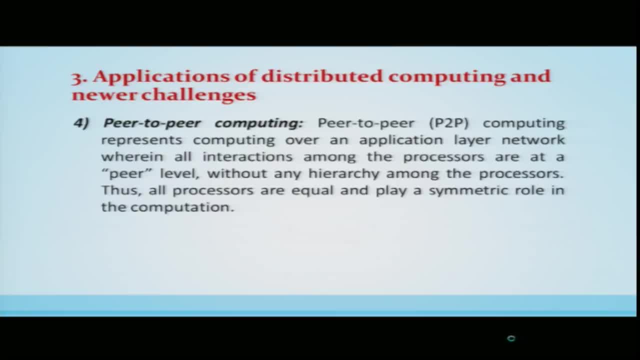 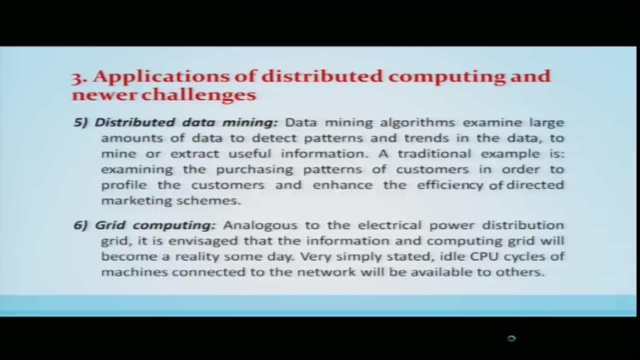 We are going to touch upon later on in this part of the course. Distributed data mining is another application of a distributed computing, So distributed data mining. Distributed data mining algorithms examine large amount of data to detect the patterns and trends in the data to mine or exact useful information. 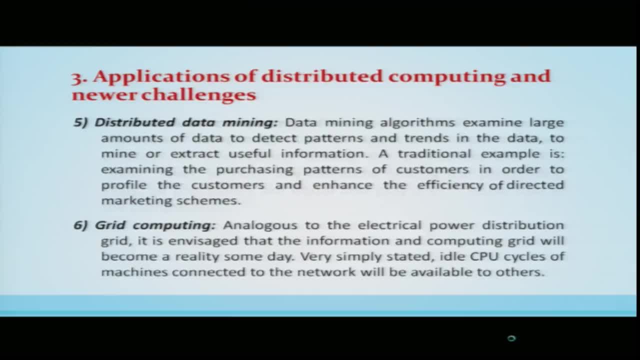 The traditional example is examining the purchasing patterns of the customer in order to profile the customers and enhance the efficiency of the directed marketing schemes. Another application of a distributed computing is find in the grid computing Distributed computing. Distributed computing, The grid computing analogous to the electrical power distribution. 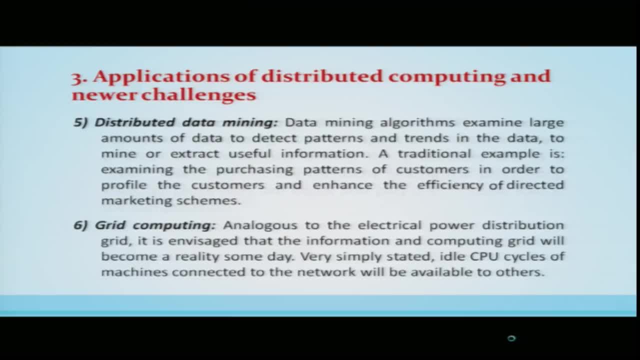 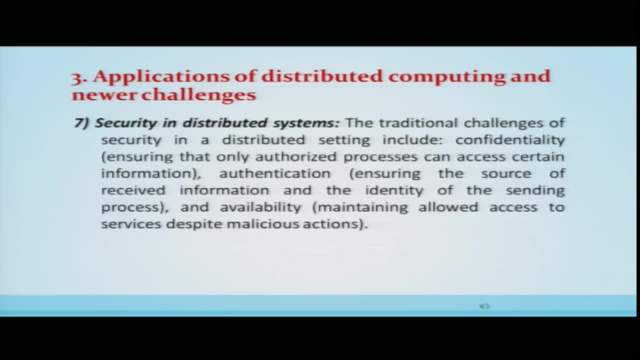 Grid. it is envisaged that information and computing grid will become a reality someday. Very simply stated, idle CPU times of the machines connected to the network will be available to the others. Another application is the security in the distributed system. The traditional challenges of the security in a distributed setting include confidentiality. 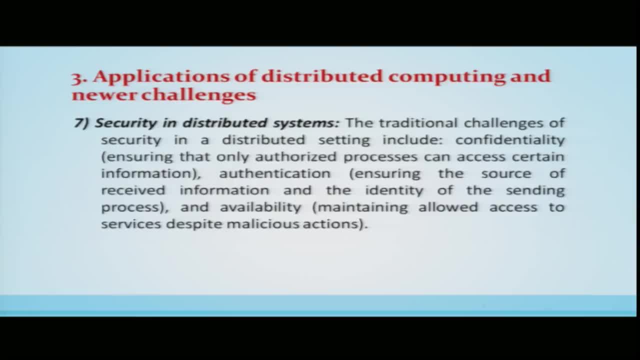 That means only authorized person can access. Confidentiality means ensure that the source receive the information and the identity of the sending process are basically the genuine and availability is the maintaining allowed access of service despite malicious actions. So security in a distributed system is used in the payment systems, the online purchasing. 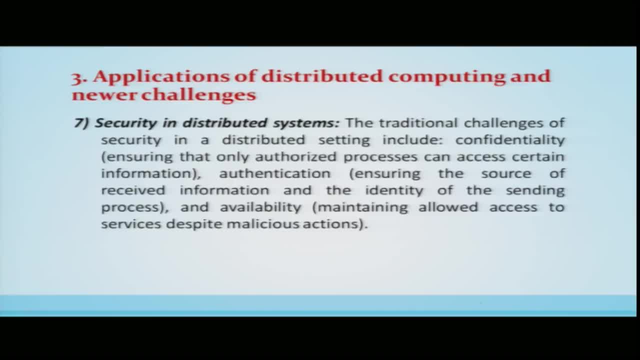 and also the recent Bitcoin. that is, the digital money. how the digital money is realized, lot of security. Next slide, please. algorithms are involved in a distributed setting, So we are going to cover up this aspect also and basically this is important because in 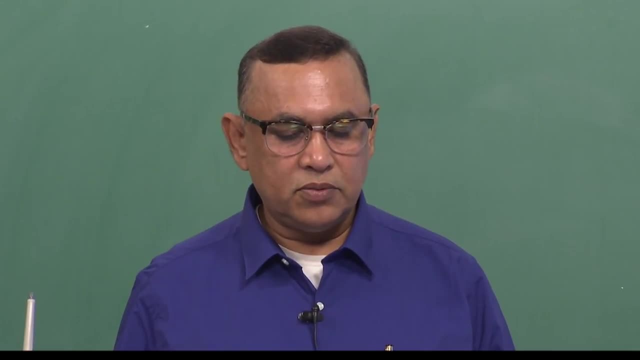 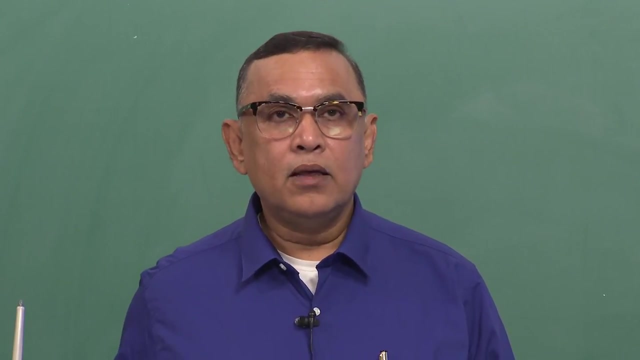 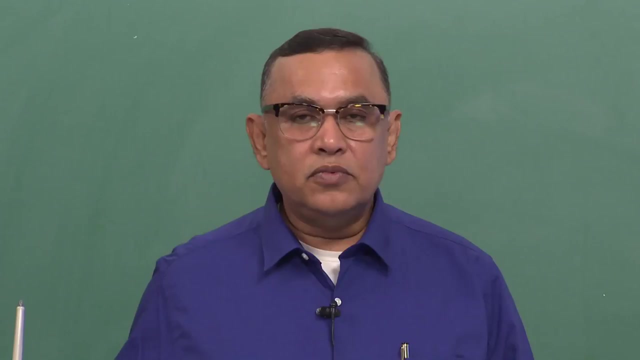 the financial market. this is most of the. this is one of the most important factor in designing such applications in the distributed systems. So, in the nutshell, what we have seen here is the distributed systems as having a wide variety of application real world scenarios, and some of them we have covered up in this. 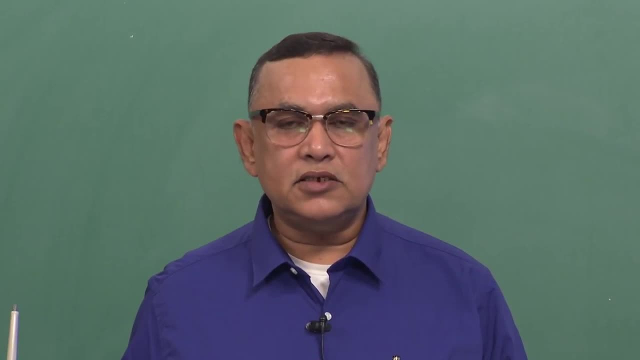 part of the introduction and this will be the basis and of understanding or pinpointing or underpinning the intricacies, the theoretical and intricacies to understand the reasoning, how the things are being designed and evolved and also we can verify the its correctness, that it is correctly working.